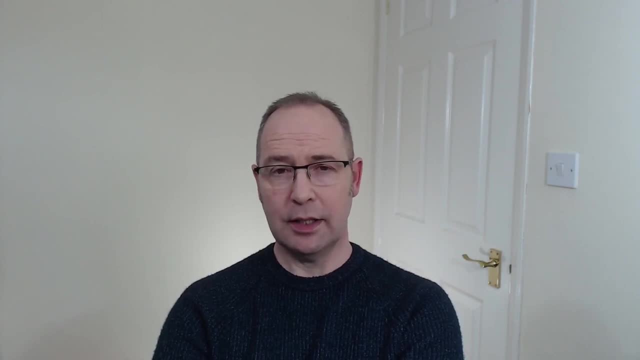 Networks enable computer devices to communicate, and as IT professionals, we're responsible for configuring those networks and also troubleshooting them too. When it comes to troubleshooting, the ping utility is one of the most useful tools that we have at our disposal Now. the ping utility is something that is often underused and sometimes misunderstood. I'm sure many of you have used it. 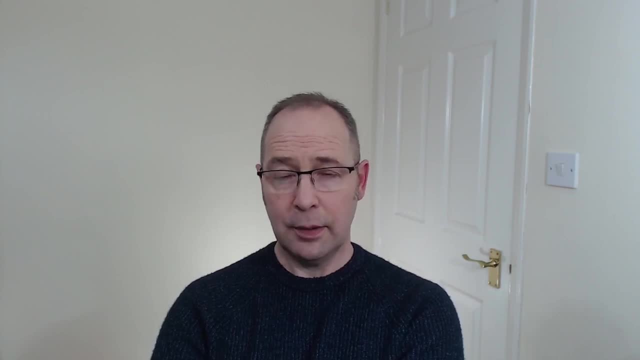 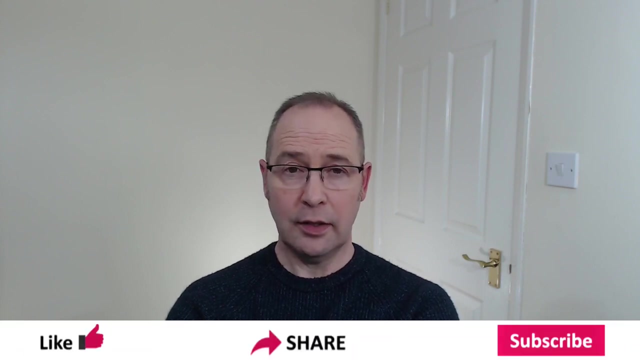 already, but in this video we're going to take a closer look at ping, and I've also included some additional information to help those of you studying for network certifications like CCNA or Comtia Network Plus. Now, before we get started, please help the video by giving it a like. 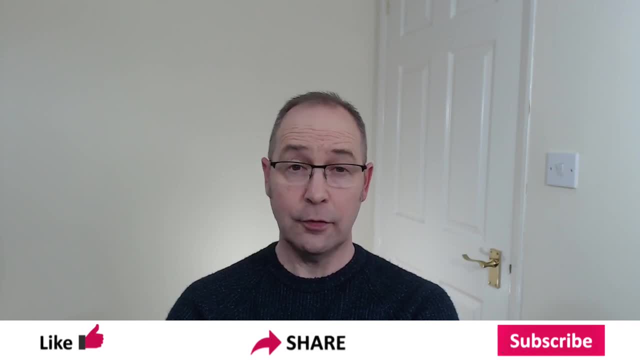 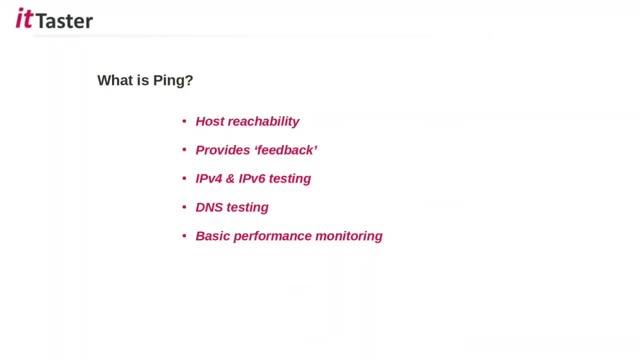 share it, and don't forget to subscribe to the IT Taster channel for new content. Okay, let's get into the video. The main reason we use ping is to test if we're able to reach a remote host on an IP network. Are we able to contact that host Now? this could be a PC. 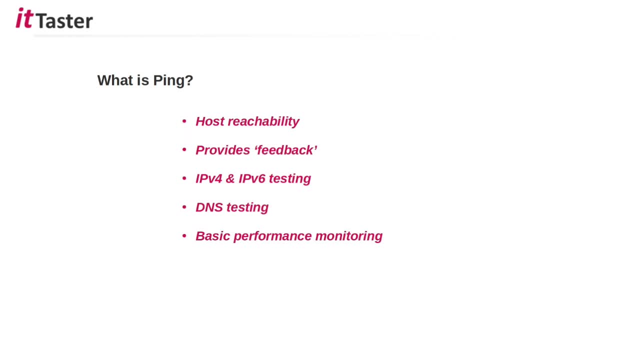 a server, a network switch or a router, for example. Now, ping's job is to provide us with information feedback, and this makes it incredibly useful for diagnosing network issues. We could use it to test IP version 4 and IP version 6, as well as things like DNS. 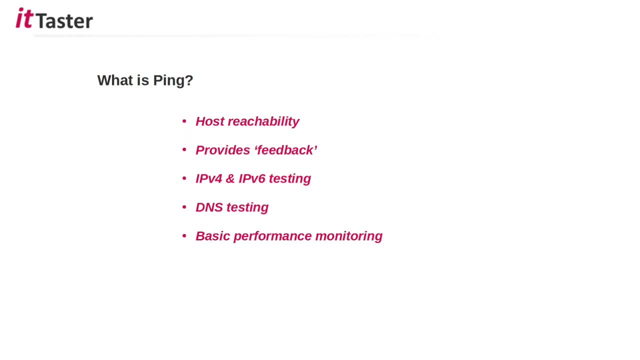 Ping can even be used for basic network performance monitoring. Now, an important point to note is that ping is a utility, a tool. It's not a network protocol, but sometimes this can be misunderstood. Now, in order to learn about how the ping utility works, we need to begin by looking at the Internet. 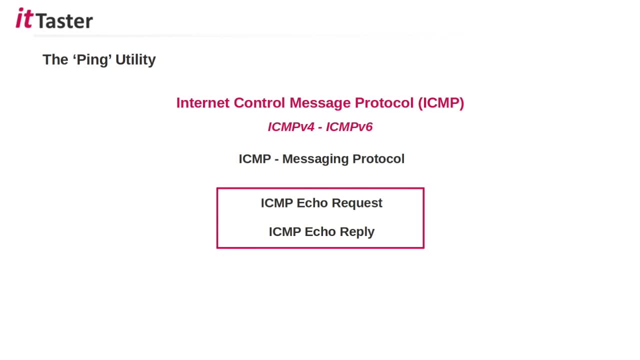 Control Message Protocol, ICMP. There are two versions of ICMP: ICMP version 4 for IP version 4 and ICMP version 6 for IP version 6.. Now the ICMP version 6 is a protocol that is used to stop a remote host from being able to reach a remote host on an IP network. Now, ICMP version 6. 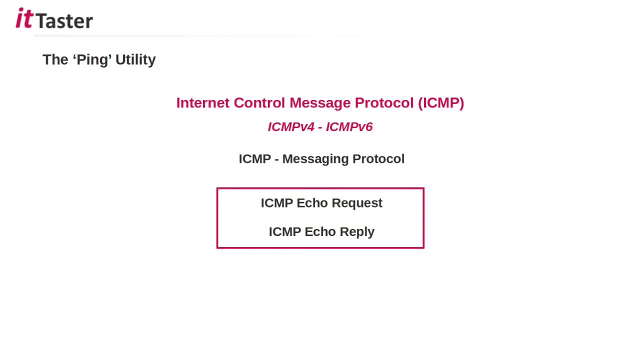 also has additional functionality which is outside of the scope of this video. Now, ICMP is a messaging protocol, and two of its message types that are really useful are the echo request and echo reply messages. The ping utility uses these to determine if a host is reachable. 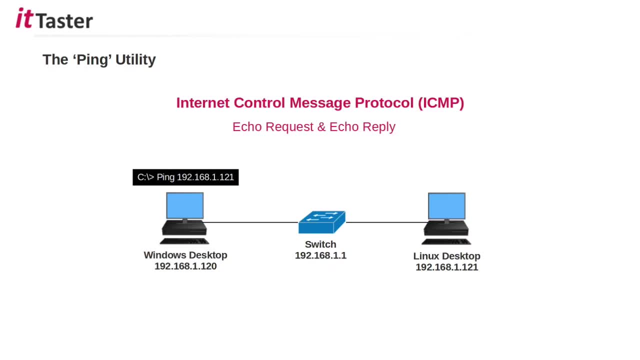 In this example, the ping command is run from the Windows desktop to ping the IP address 192.168.1.121,, the IP address of the Linux desktop. An ICMP echo request is sent to the Linux desktop and when the Linux desktop receives the echo request, it responds by sending back an echo reply. Now, 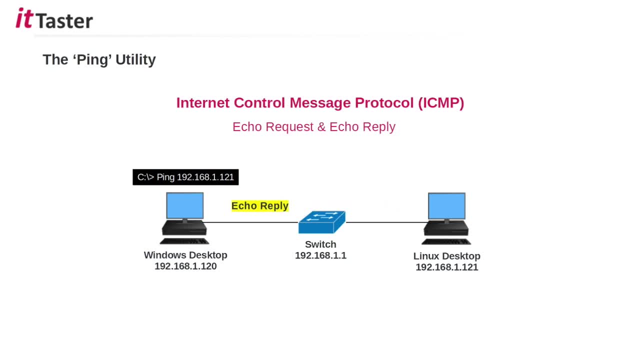 when ping is run on a Windows desktop. this process takes place four times by default and we'll see this in action later on in the video. It's sometimes helpful to think of the echo request and echo reply process as the source host. 192.168.1.120. asking: are you there? 192.168.1.121. 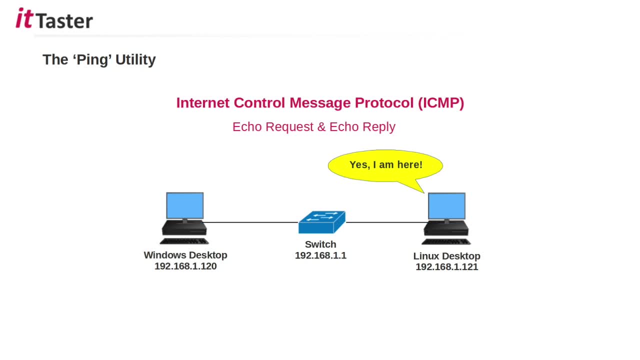 and the destination host replying: yes, I'm here Now. things in the world of IT don't always go accordingly. Now in this example, we have a network switch failure. The Windows desktop tries to send an ICMP echo request to the Linux desktop. The echo request isn't received by the Linux desktop and 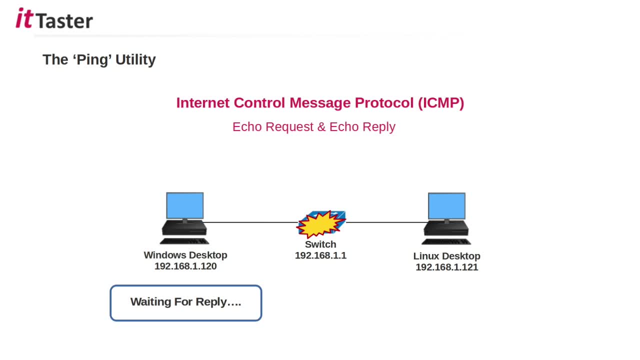 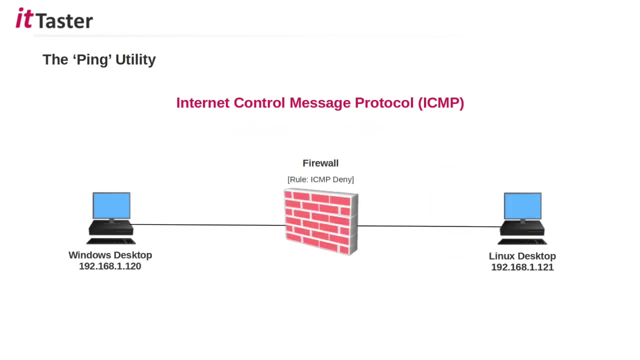 therefore, it's not going to send an echo reply. The ping utility will wait for an echo reply until the timeout value is exceeded. Ping will provide us with feedback to indicate this. for example, requests timed out Now. it's important to be aware that firewalls are typically configured to block ICMP for security. 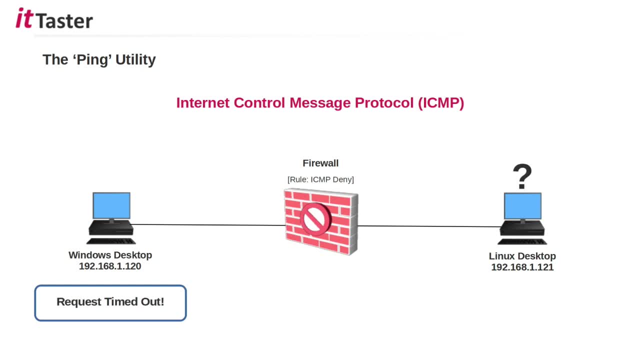 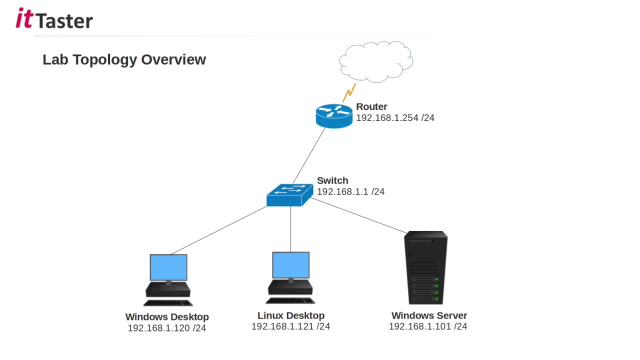 reasons, and this will prevent ping from working as expected. Therefore, when carrying out diagnostics using the ping utility, keep in mind a firewall could be blocking ICMP traffic and could be the reason ping isn't receiving a reply. This is a diagram of the lab setup that I'm going to be. 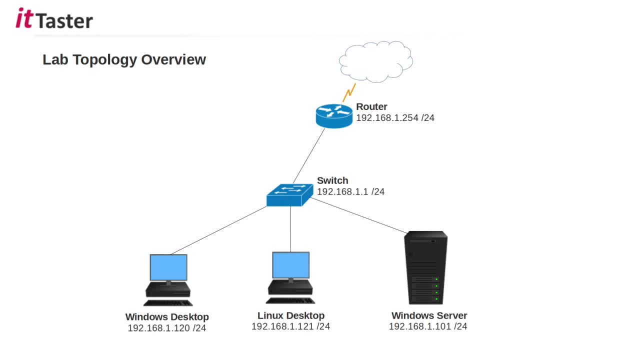 using to show you the ping utility in the next video. Thank you for watching and I'll see you in the next video. Ping utility in action. We have two computer workstations. We have a Windows desktop and a Linux desktop. We have a Windows server, a network switch and an internet router- the default. 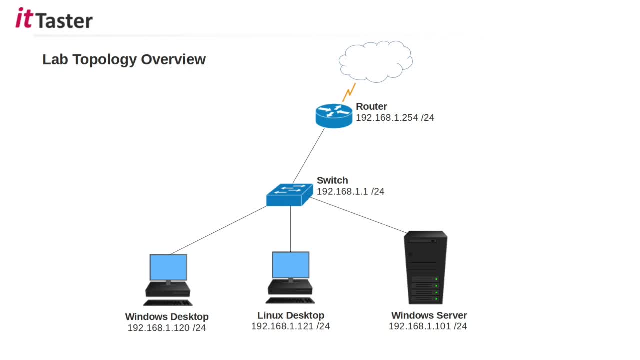 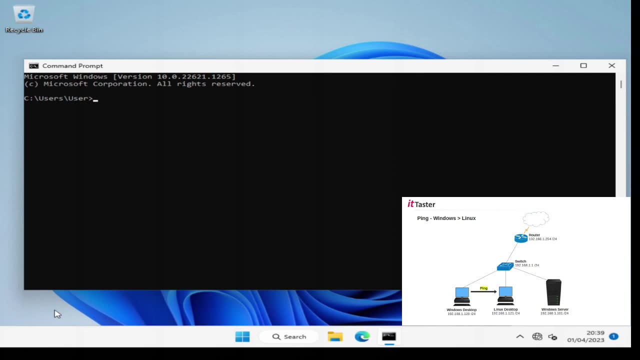 gateway. So let's get into the lab and start working with the ping utility. I've switched to the Windows computer in the lab and I'm going to begin by pinging the Linux computer. To do that, I need to type the command png, followed by the IP address of the Linux computer, which is 192.168.1.121, and hit return. 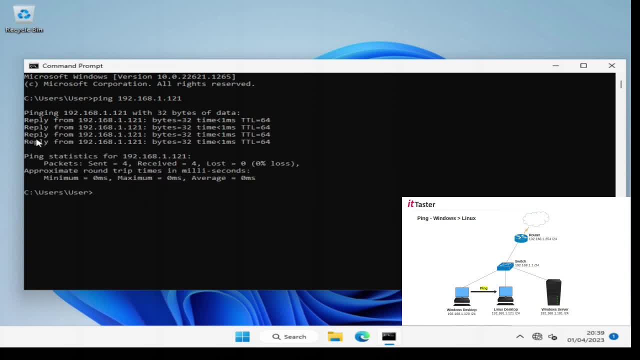 Now, as you can see, we're already receiving echo replies, which tells us that the Linux host is reachable. We also have some useful information included within this as well. We can see the things like the round trip time. This is the time taken to send the echo request. 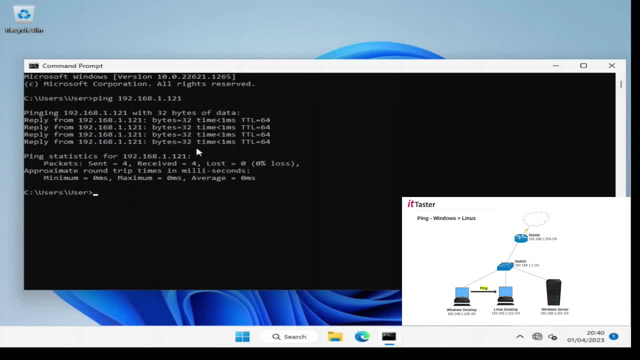 and receive a reply And, as I've already mentioned, Windows does this four times by default And we also see a summary below. We can see that we sent four packets, we received four replies and we lost zero packets, zero percent loss. We can also see the approximate round trip times. 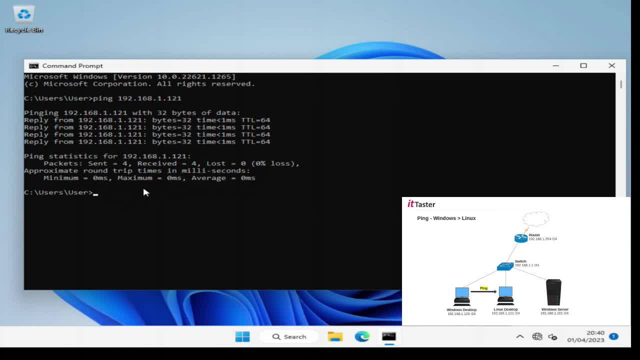 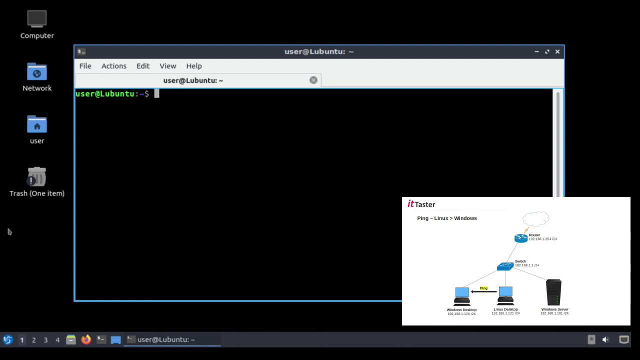 below here as well, and the average as well. So let's now go over to the Linux computer and run ping utility from there to see what that looks like. This computer is running Lubuntu, Linux, and I'm going to try to ping the Windows computer from here. To do that, we just type the ping command as: 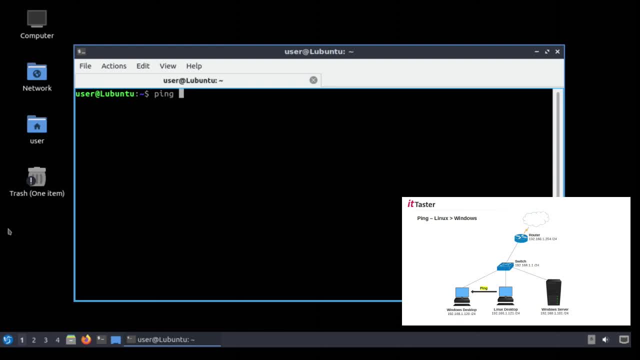 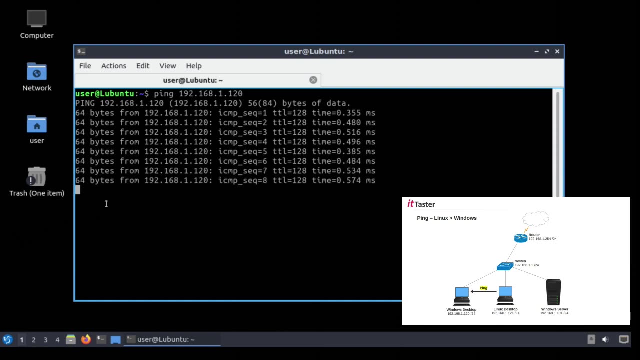 before, followed by the IP address of the Windows computer, which is 192.168.1.120, and hit return. Now the first thing you'll notice is that Linux sends a continuous ping. So if we need to stop it, we just need to hit control and C on the keyboard. 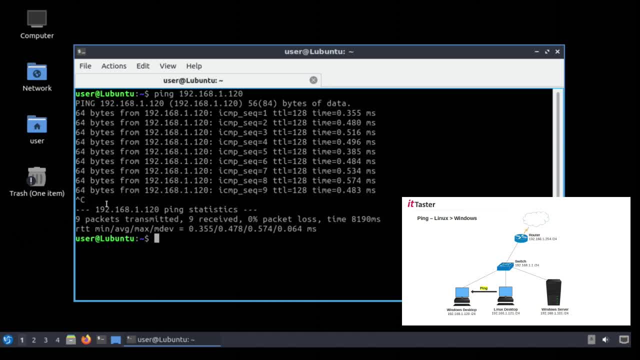 Now, if we don't want a continuous ping in Linux, we can use the minus C switch, followed by the number of pings that we want to send. So let's give that a try. Let's type: ping minus C. I'm going to choose 4, so it looks like the Windows version of the command and the IP address of. 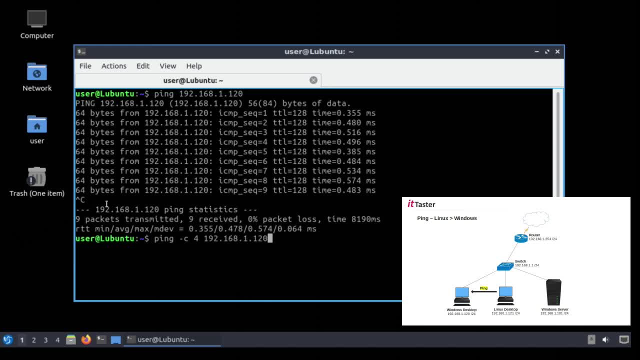 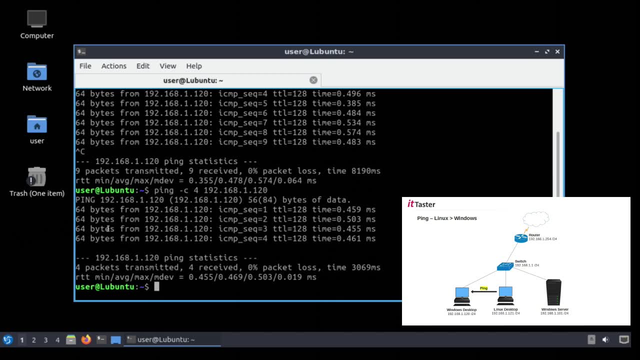 the Windows computer again and hit return. Now, as you can see, we're successfully receiving echo replies, which tells us we're able to reach the Windows host too, And, just like the previous example, using Windows we have some useful information. We have the IP address. the echo replies are received from the protocol we can 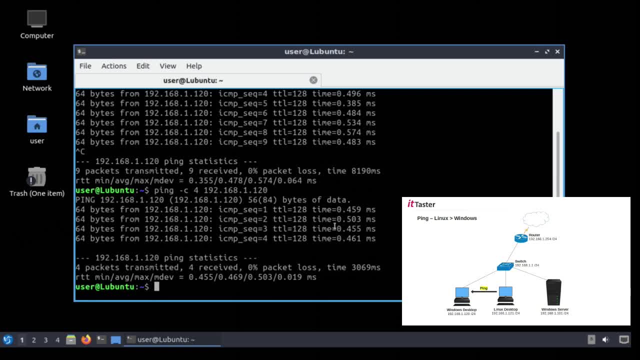 see ICMP. the round trip time is here as well, and the same useful summary below. We sent four packets, received 4 and 0% packet loss. Now many devices like switches and routers also include a ping utility, So let's see what happens when we try to ping the Windows computer using a Cisco. 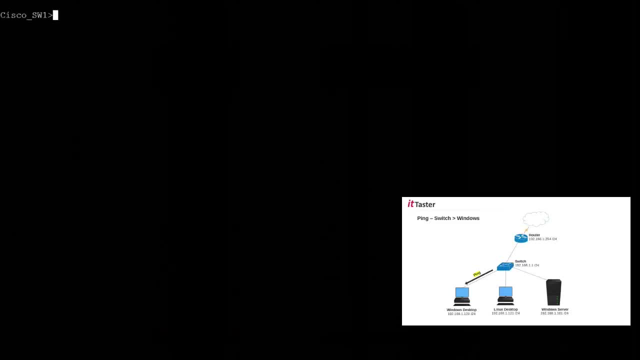 managed switch. This time I'm connected to a Cisco managed switch using the console port and I'm using Cisco iOS, which is Cisco's operating system. So let's begin by trying to ping the Windows again. To do that, all we need to do is type ping, followed by the IP address of. 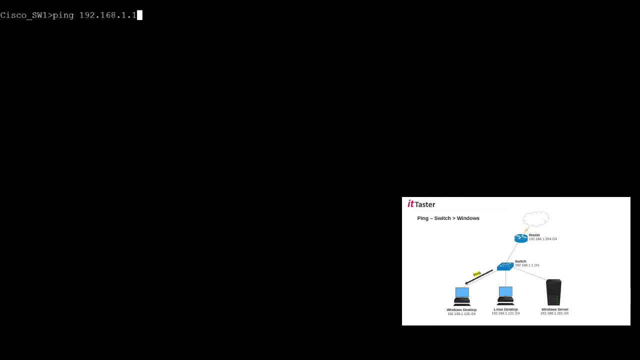 the computer, which is 192.168.1.120.. Hit return and the first thing you'll notice is that ping responds a little differently to what we've seen so far. On the Cisco switch we receive an exclamation mark to indicate a successful echo reply. In fact, we have five exclamation marks indicating five. 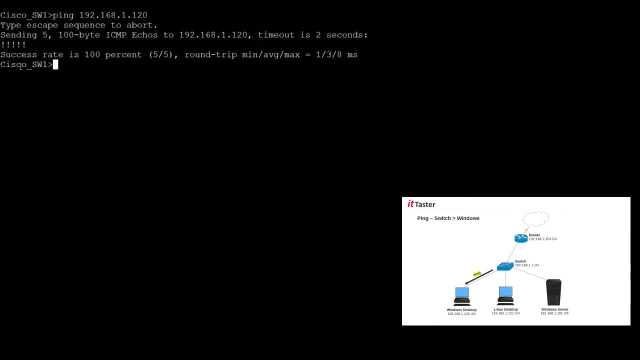 successful replies, and we also have a summary below telling us the success rate is a hundred percent: five out of five. Now the next thing I want to do is just disconnect the Windows computer temporarily and ping its IP address again so that we can see what happens. The Windows computer is now disconnected. 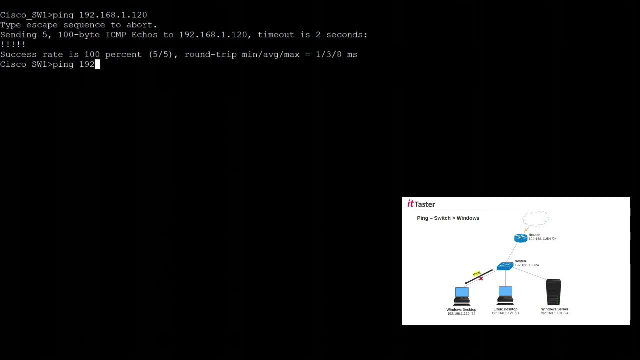 so let's try pinging it again Now. the first thing you'll notice is that the response is much slower, and this is because ping is waiting for the echo requests to time out. You'll also notice that we receive a dot to indicate time expired. We're unable to contact the 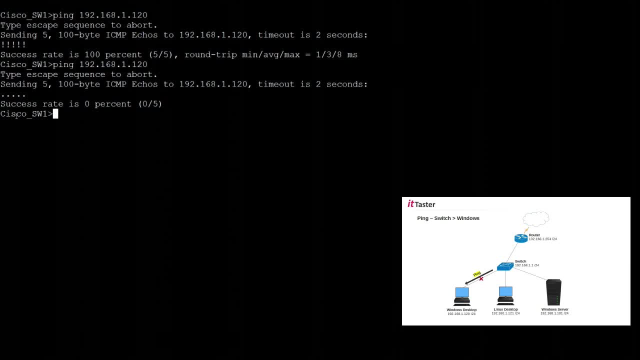 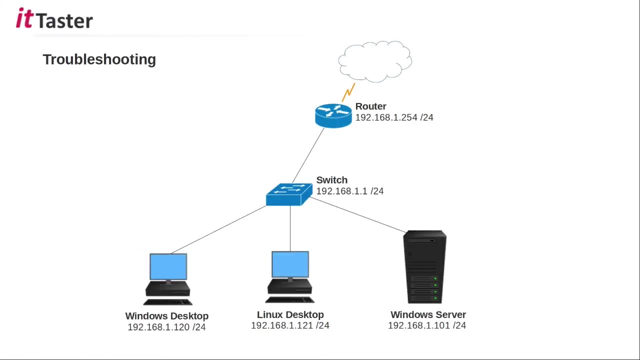 device, and the summary below also indicates this. as you can see, the success rate is zero percent, zero out of five. Now it's really important to know how ping works from Cisco devices, especially if you're studying for your CCNA. When we use ping to troubleshoot a 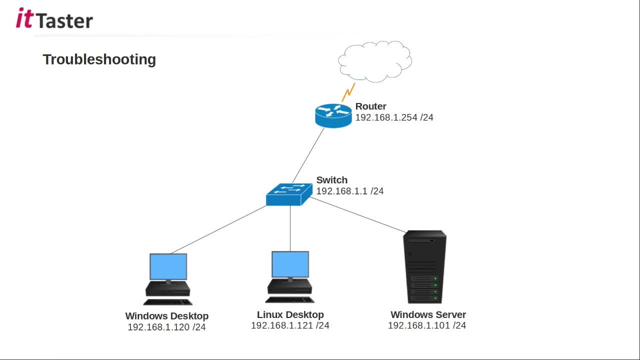 network issue. it's a really good idea to follow a logical process, and the first place to begin the diagnostic process is to test the local device first. so I'm going to use the Windows computer again for this. Now there's a special IP address set aside for us to use to test the local device. 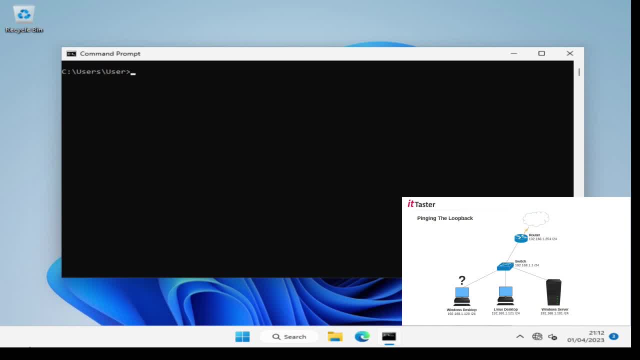 device, and this is called the loopback address. Think of this address as itself. Now, this is an important address to remember, especially if you're studying for CCNA or Network+. Now, the loopback address for IPv4 is 127.0.0.1.. The loopback address for IPv6 is: 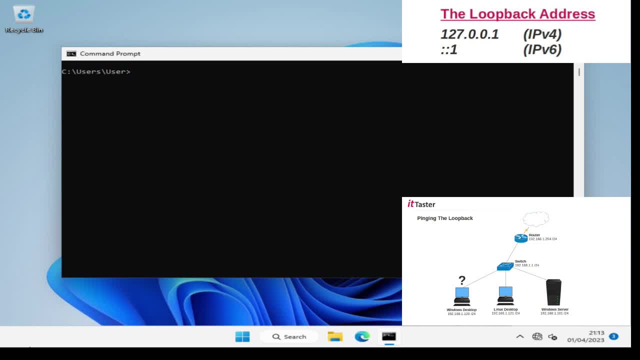 colon, colon 1.. So let's give them a try. I'll ping the IPv4 loopback address first. As you can see, we're getting a reply. response from the IPv4 loopback address. Let's now ping the IPv6 loopback address. 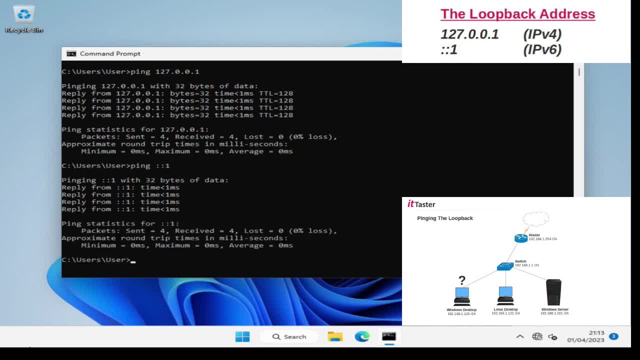 Again, we're also getting a reply- response from the IPv6 loopback address, which is good. However, this is a really important point to remember: When you're doing a loopback loop, it's important to remember that all the pressing and closing 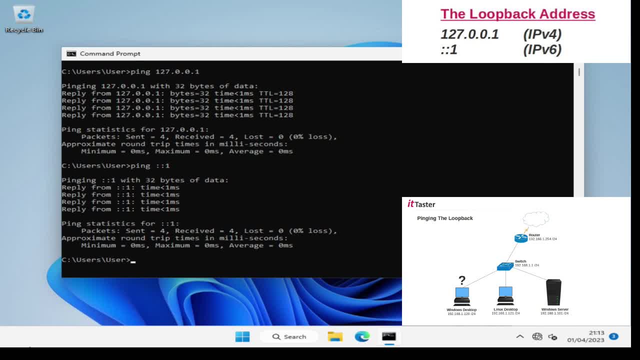 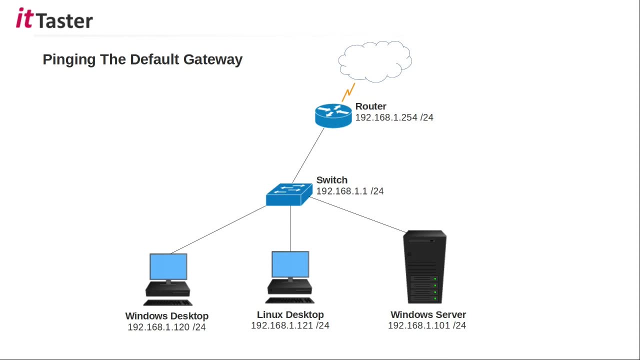 when we ping loopback addresses. this is a very limited test. it only tells us that ip is correctly installed on the local device. it doesn't test beyond this. it doesn't test the network card or cabling, etc. okay, after we've successfully pinged the loopback address, the next step is to 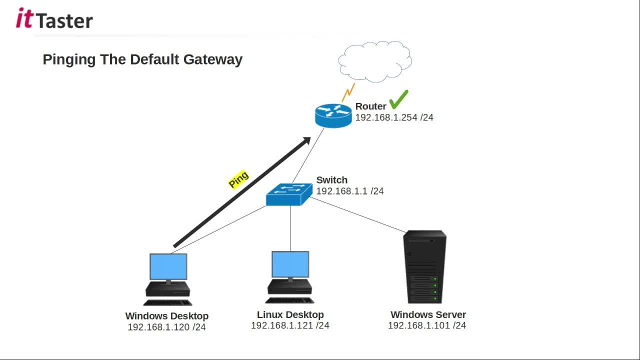 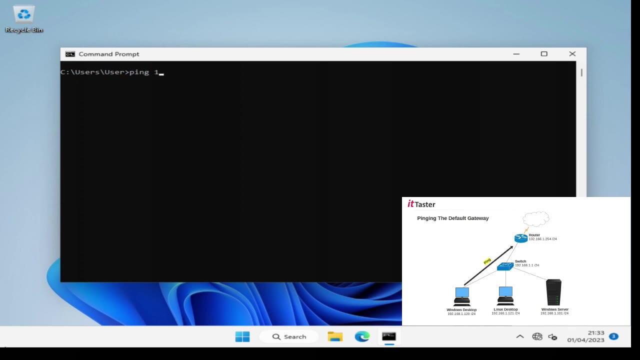 ping the default gateway, the router, because if we're able to successfully ping the default gateway, we should be able to talk to the other devices on the local network. so let's just quickly check that we're able to ping the default gateway. okay, so ip address is 192.168.1.254. 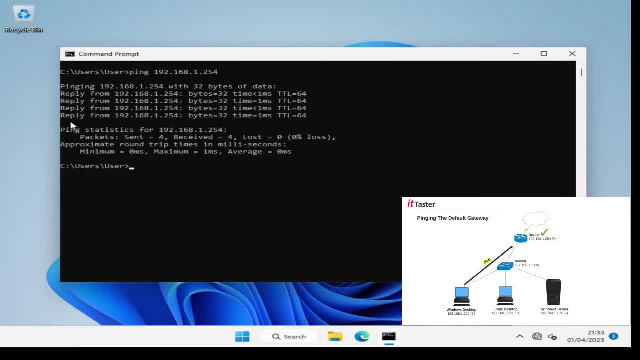 and, as you can see, we are successfully receiving echo replies. so all is good there and we should be able to talk to the rest of the local area network now. the next step in the process would be to ping a remote host on another network to verify connectivity beyond the local network. 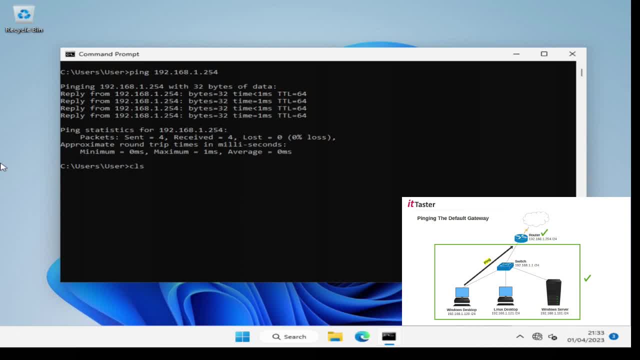 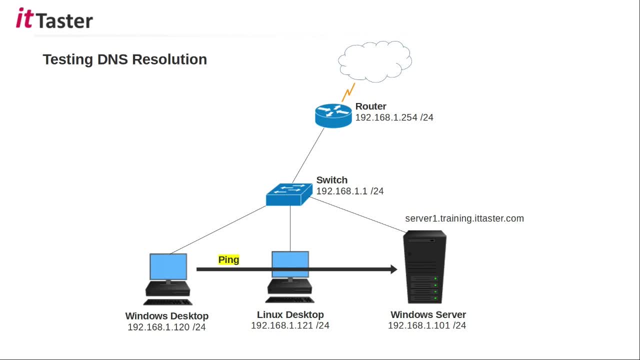 but i'm going to leave the diagnostic process there now. the ping command doesn't only ping ip addresses, we can ping host and domain names too. this means that ping can be used to test dns resolution, and this is because ping must first query a dns server to resolve host or domain name in order to ping its. 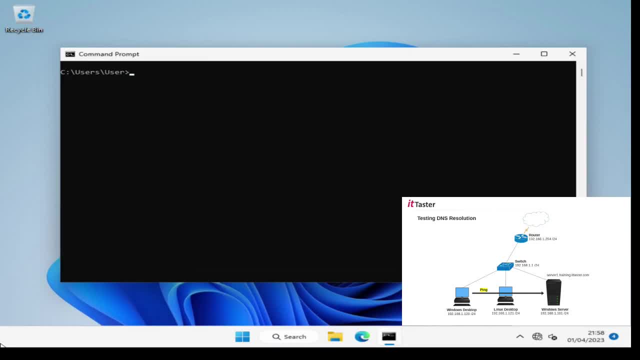 ip address. so i'm going to ping the windows server in my lab using its dns name type, ping minus 4, and the minus 4 switch, by the way, tells ping to use ip version 4 only. and then my server name, which is server1.trainingittastercom. 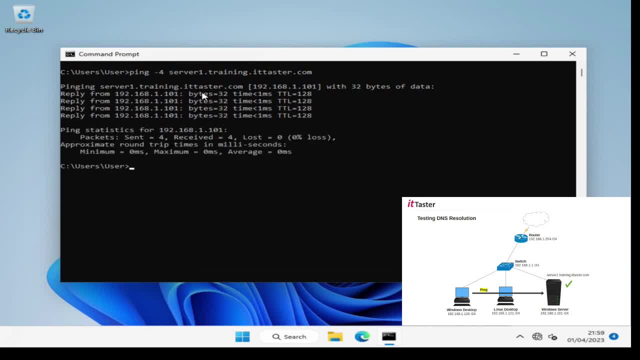 we can see here the host name server1.trainingittastercom is resolved to the ip address 192.168.1.101 and that tells us that dns resolution is working okay. we can also see our echo replies and the usual summary below as well. 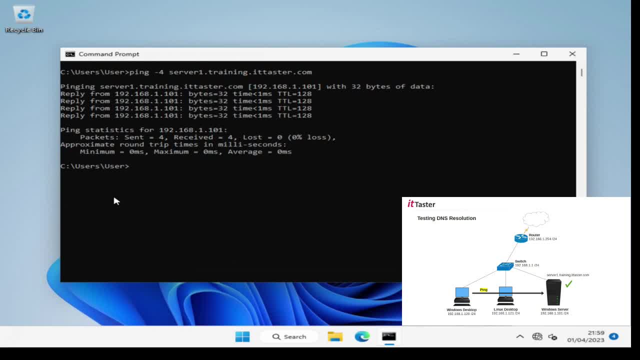 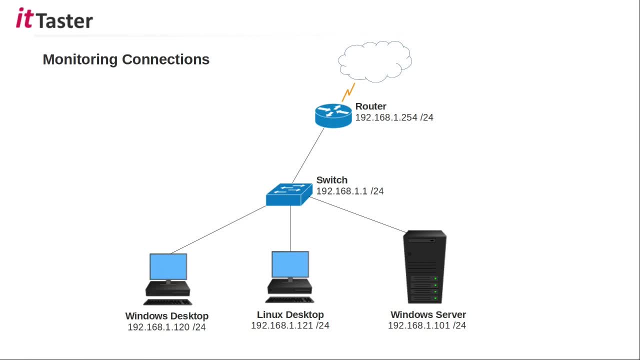 so we can use ping to combine two tests here: to quickly test dns resolution and also check if we're able to contact a host. a useful diagnostic technique i want to show you next is how the ping utility can be used to monitor connection issues, for example where 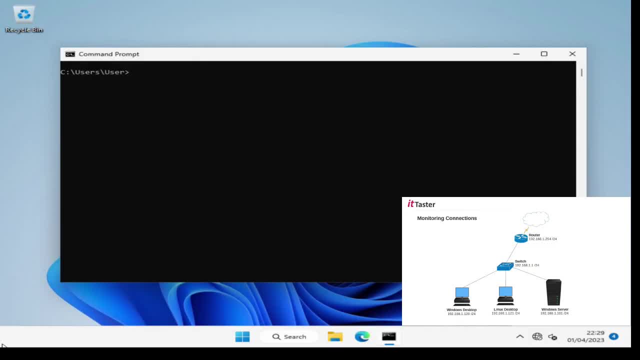 there is an intermittent fault. now to do this i'm going to use a continuous ping. now, as you've already seen earlier in the video, linux does this by default, but in windows we need to use a switch. the switch to do that is minus t. minus t basically means ping until stopped and the ip address that. 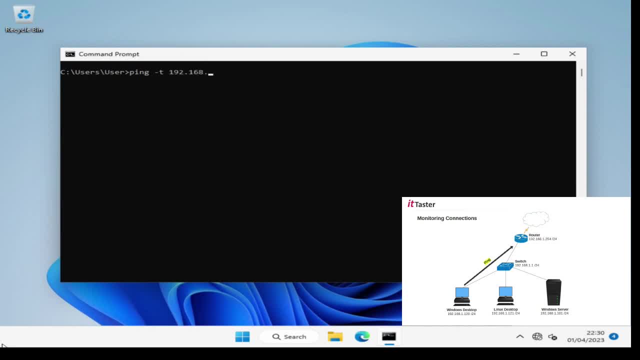 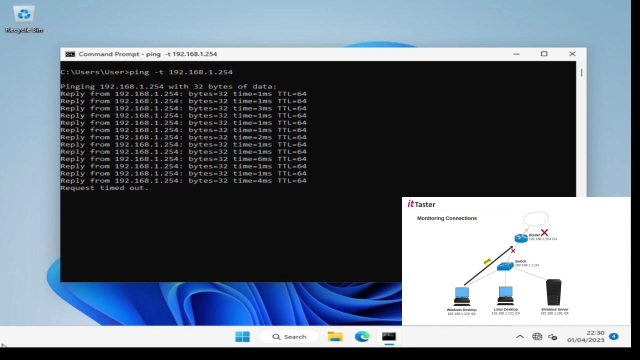 i'm going to use is my default gateway, again 192.168.1.254. now, as you can see, we begin to receive lots of replies. so now i'm going to simulate an issue by disconnecting my default gateway. now, as you can see, we're starting to receive requests, timed out messages indicating that we're 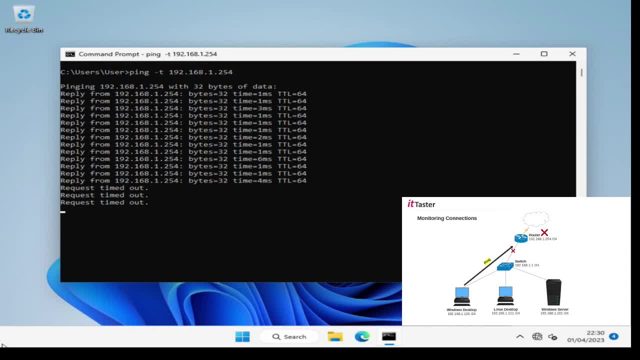 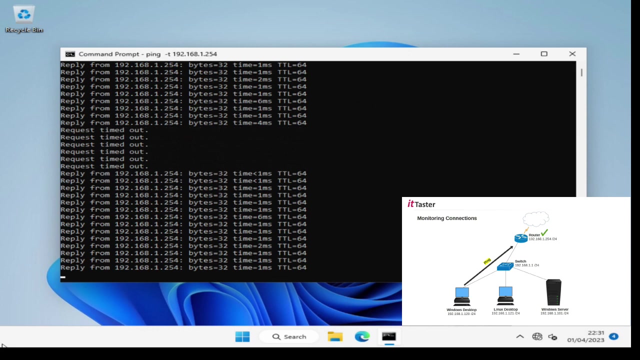 indicating there's a problem here. I'm now going to reconnect my default gateway again and we receive replies again. This can be a really great way to monitor connections and connection issues. Now to exit the continuous ping, all we need to do is press ctrl and c on the. 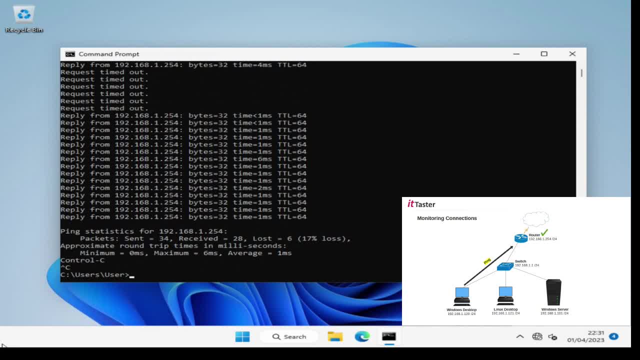 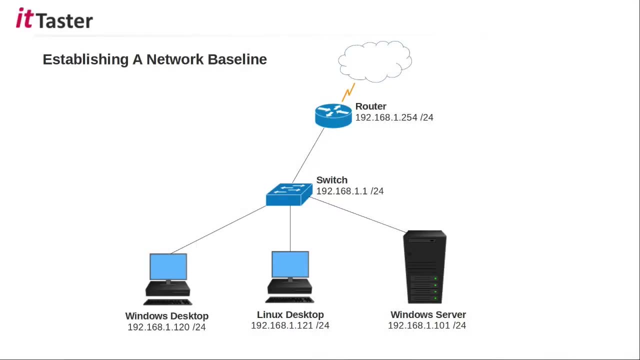 keyboard. Incidentally, if you try a continuous ping using a wireless connection, you'll see some really interesting results, particularly in terms of the round trip times, and this is due to the way wi-fi works. I mentioned earlier in the video that the ping utility can be used to monitor performance. 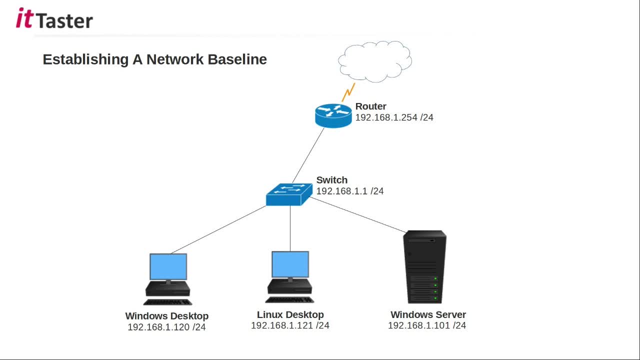 and establish a connection. If you want to see more information about the ping utility, a rough network baseline, This can be achieved by recording the feedback that ping provides us. in order to gather data about the network at various times of the day, I'm going to use a 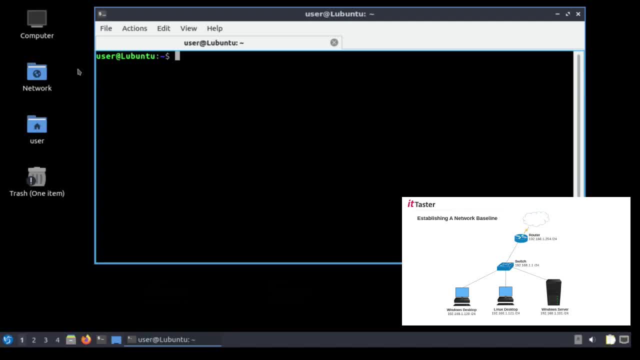 Linux desktop for this, but you can just as easily use a Windows desktop too, And in this example, I'm going to manually capture and record the information when I ping my router, the default gateway. But you can use other devices, like a server, for example. So let's ping the router. 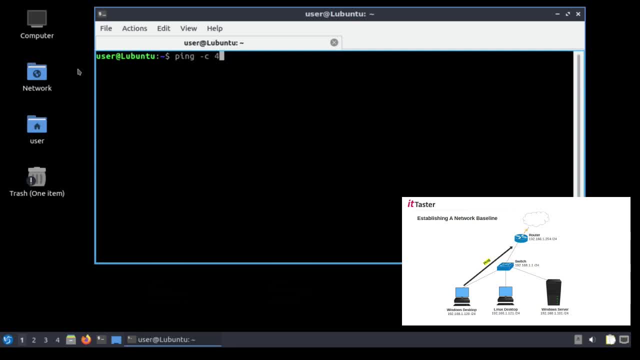 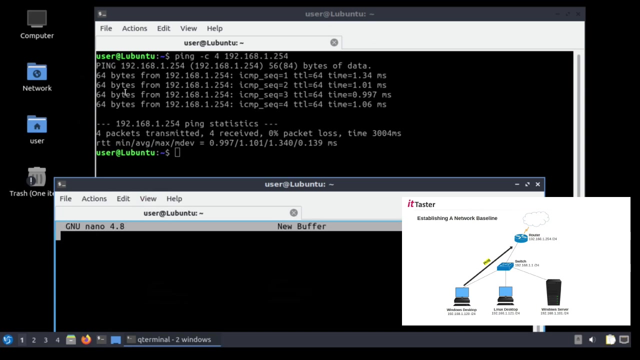 Ping Minus c. for now I'm using the minus c switch because I don't want a continuous ping for this- And my router's IP address, And we'll just let that run through. I'm just going to open a text editor. I'm going to use nano for this, And it's simply a case of just copying the information. the 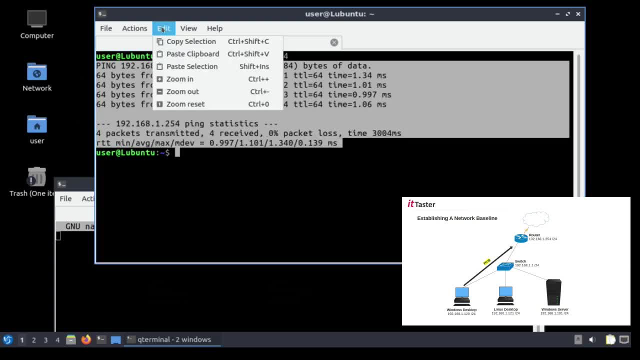 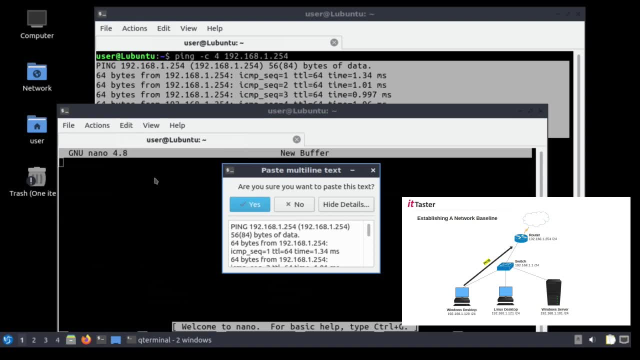 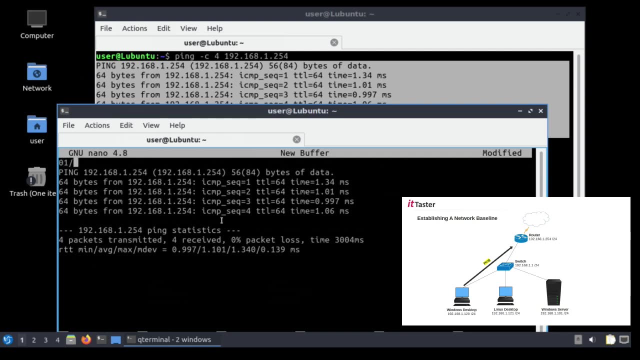 output from ping And pasting it into our text editor. Now it is, of course, very important to date and time this, So put the date in And I'm going to pretend that I captured this information at 8: 30 in the morning. 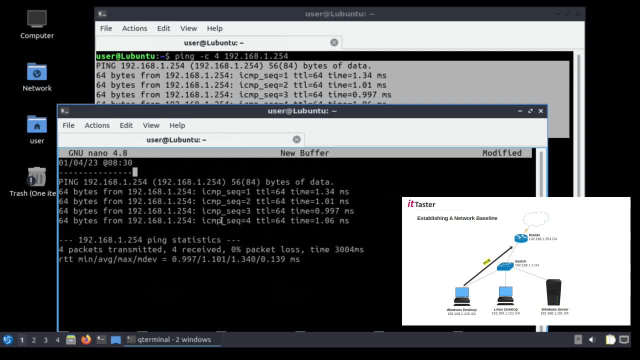 This is a good time, because many of our users will probably be arriving at 8: 30 in the morning, So I'm going to paste this in And I'm going to paste this in. I'm going to paste this in And I'm going to paste this in. 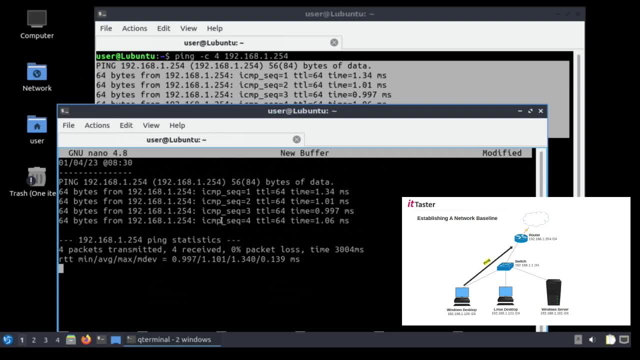 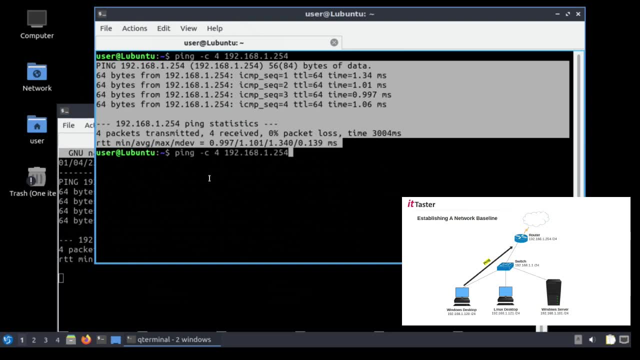 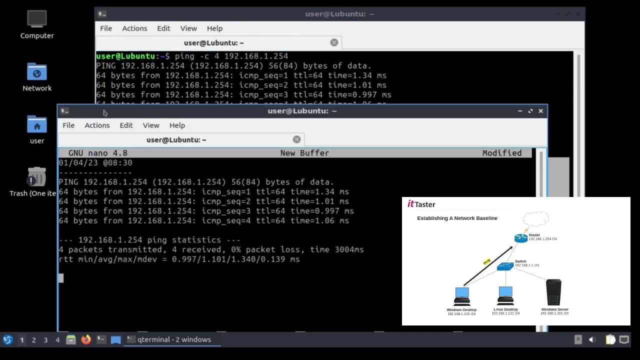 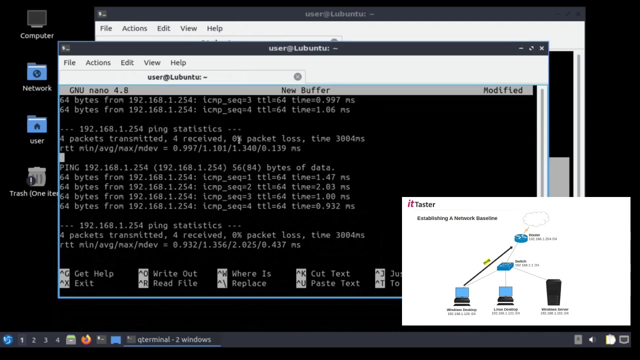 And log in on to the organization's network And then, when we've done that, we'll run the ping command. a little later in the day we'll run it again And again, copy and paste the results and remember to date and time it. and let's pretend we captured this at 11 o'clock. 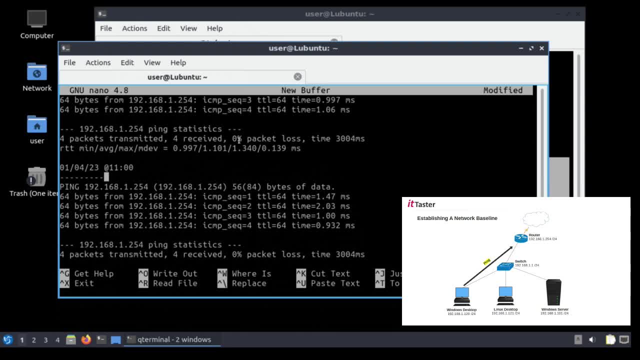 okay. so over time, this enables us to build up a baseline that we can refer back to, and it's also worth mentioning that this is something that we can very easily automate with a script. now, in order to get the most from the ping utility, it's a good idea to examine the 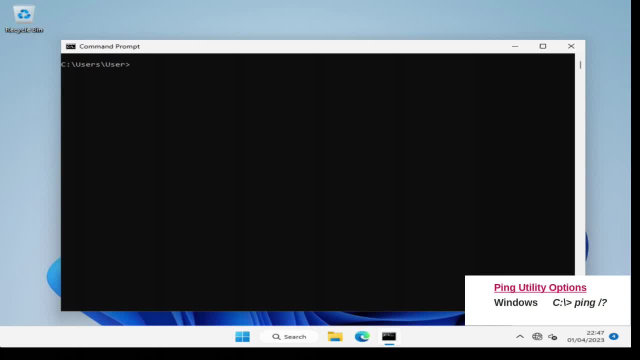 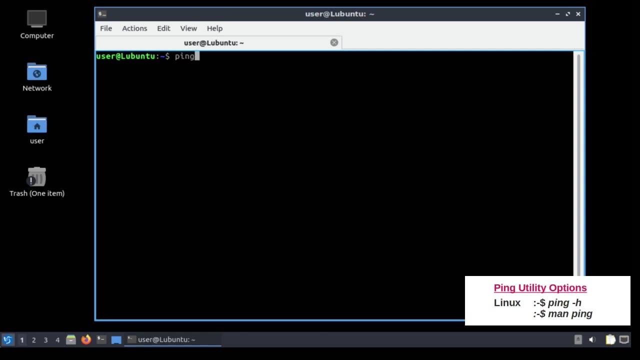 various switches available by accessing the help utility. now, to do this in windows, you can either type ping on its own or ping forward slash, followed by a question mark. on a linux computer to access the help information, we just need to type ping minus h and hit return. now, if we want. 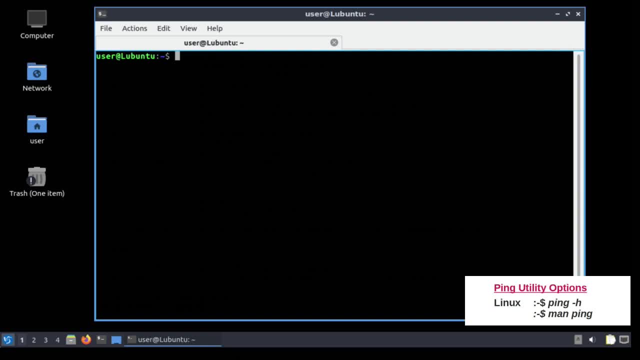 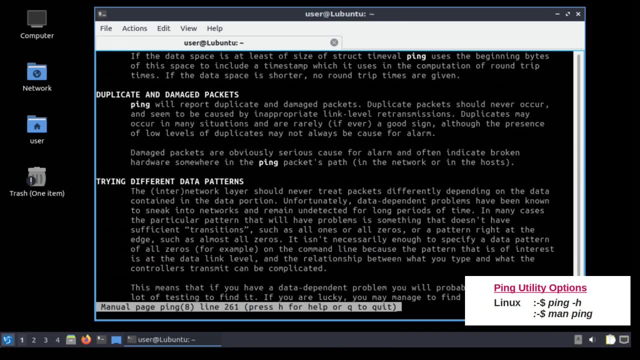 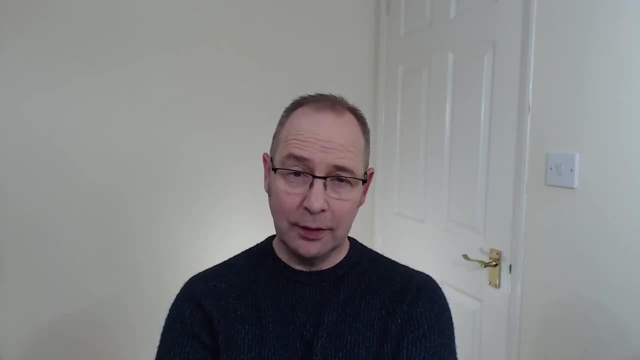 more detailed information. we can access the manual pages by typing man, followed by ping you. that brings us to the end of the video. i hope you enjoyed it. i hope you found it helpful. if you did, please give the video a like, share it and, by all means, leave a comment below. don't 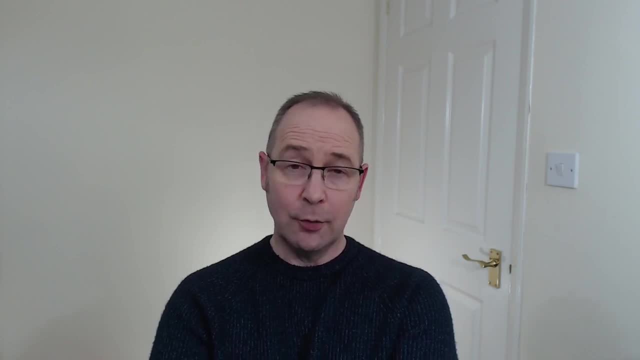 forget to subscribe to the ittaster channel too. i'm also around on social media, and the links are below in the description, so, as always, thanks for watching and i'll see you next time.